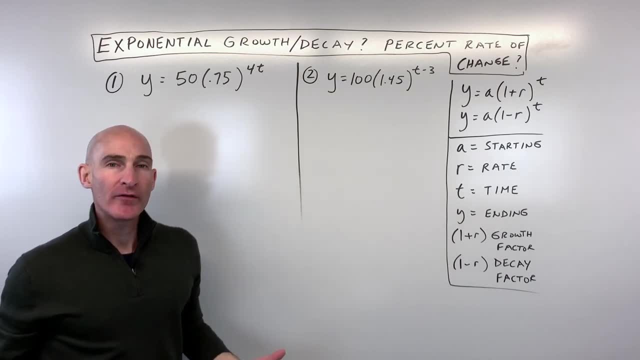 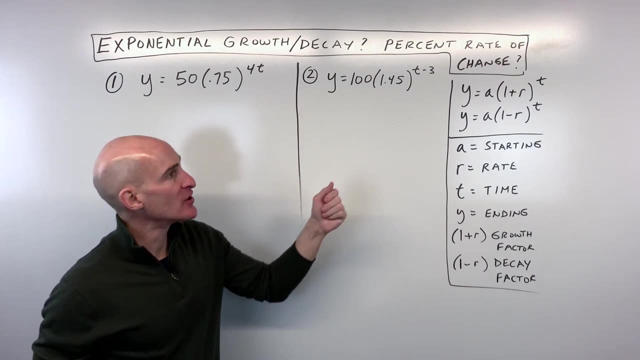 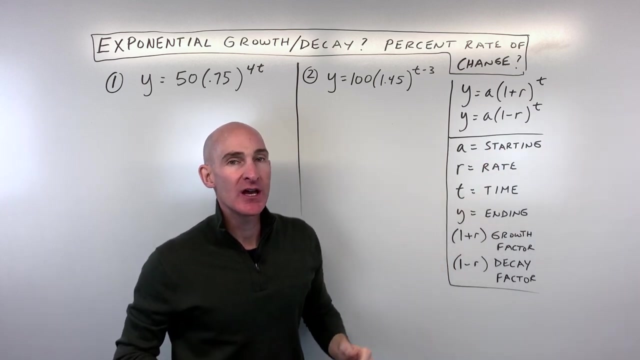 In this video you're going to learn about how to work with exponential growth functions and exponential decay functions and, more specifically, how to rewrite these equations into that exponential function form so that we can identify the percent rate of increase or the percent rate of decrease. So before we dive into these couple examples here, just a quick refresher: y equals a. 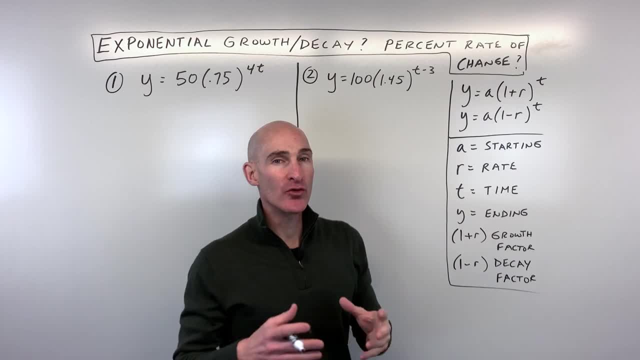 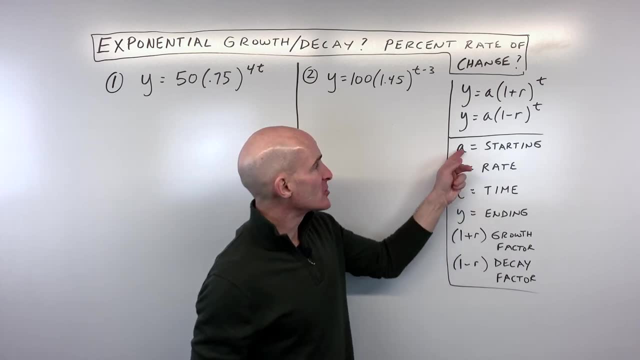 times the quantity one plus r to the t is our exponential growth function. y equals a times the quantity one minus r to the t. that's our exponential decay function. and just remember that a here represents the initial amount or the starting amount, whereas the r represents the. 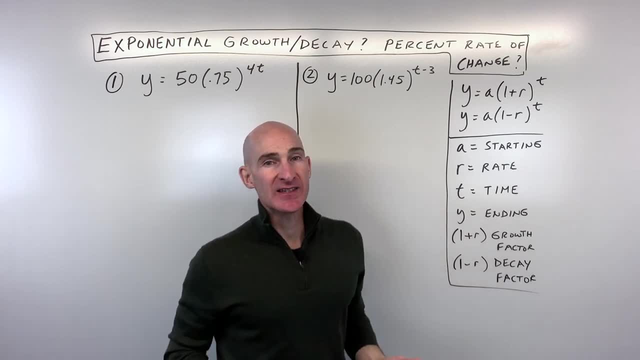 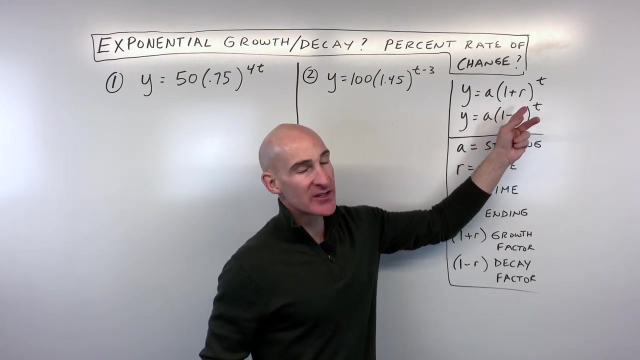 percent rate of increase or percent rate of decrease as a decimal. so you're going to have to convert that percent to a decimal. t is the time, and then y is going to be the ending amount. Now, when you look at this whole quantity here, y minus r or one one, I'm sorry, one minus r or one plus r. 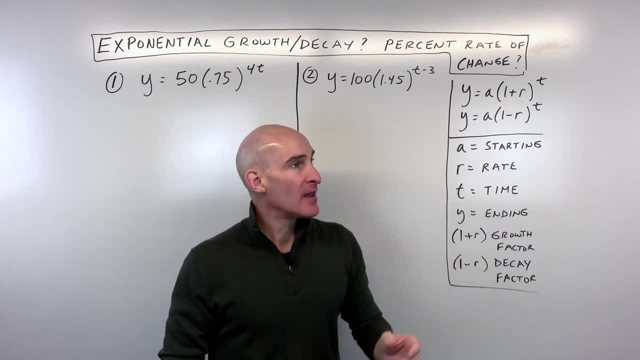 the one minus r is the time that the t is the time that the t is the time that the t is the time that represents like a hundred percent, like the original amount, and plus r means like how much more than a hundred percent. and one minus r, that r is going to be how much less than a hundred percent. 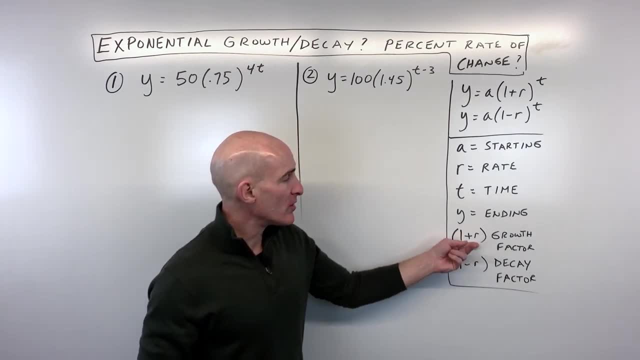 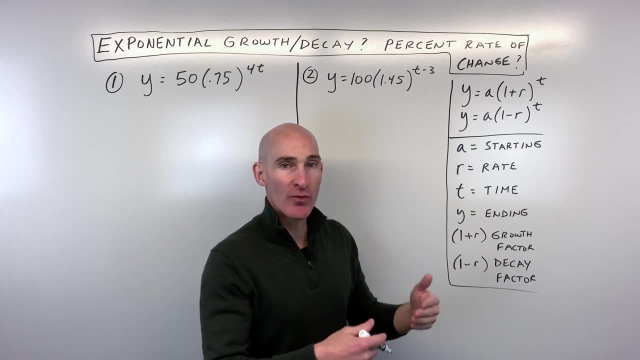 but the one is like the original amount and when you think of that, one plus r, that's the growth factor. so that's what you're multiplying by each time. one minus r is like your decay factor, which you're multiplying by each time. So let's go through a couple examples and let's talk about 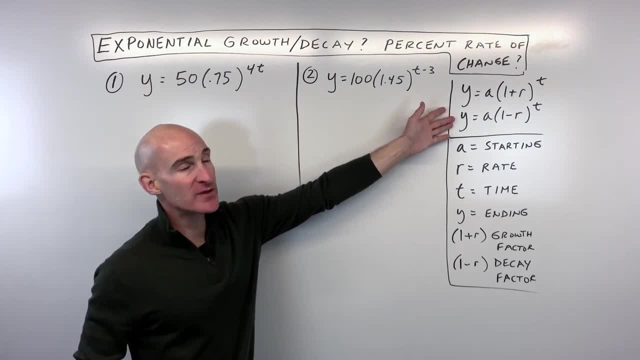 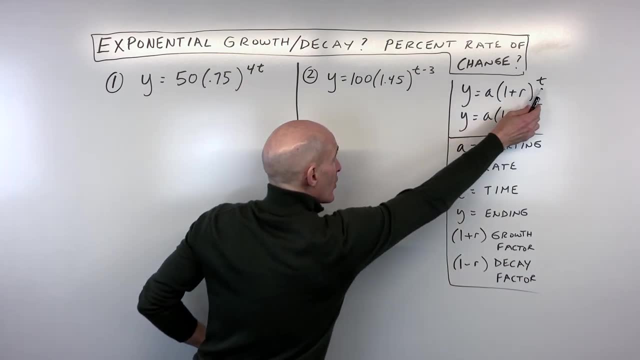 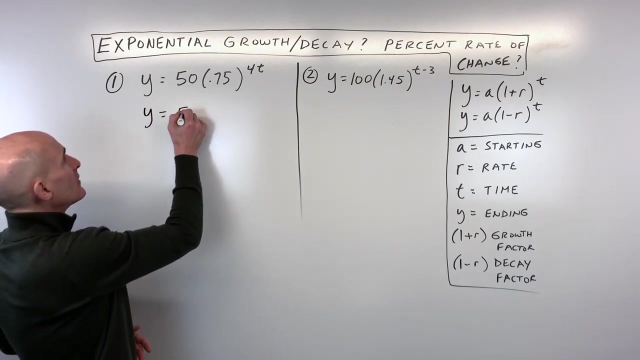 how to rewrite these so that they match these forms here. So in this first example you can see is we've got this: 0.75 to the 4t, not to the 1t. so how can we rewrite that? well, we're going to use our rules of exponents and the way we're going to do that is we're going to say 0.75. 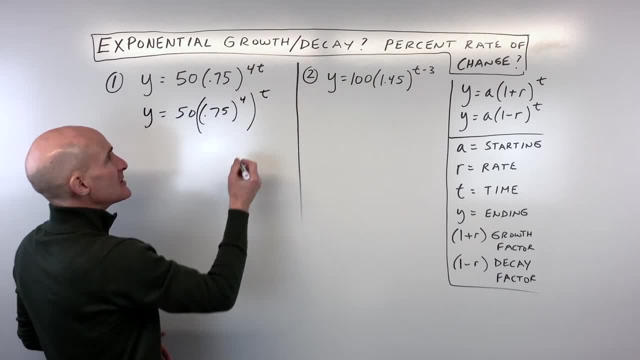 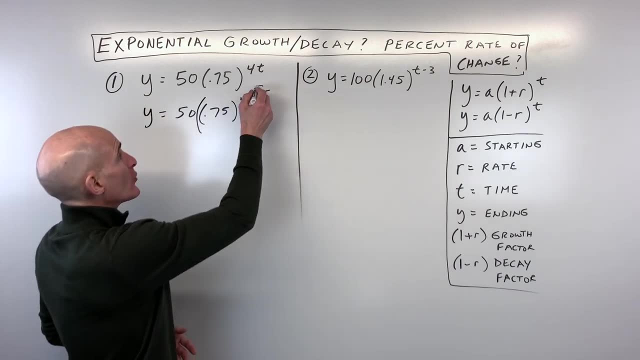 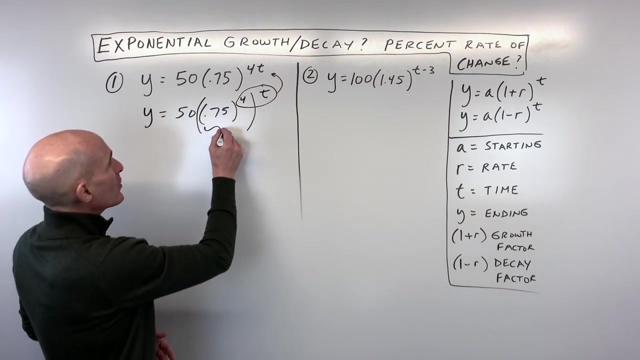 to the fourth, all raised to the t power. because remember, when you have a power to a power or an exponent raised to another exponent, what do you do? you multiply those exponents, and that's going to give us back our original equation. But now what I'm going to do is I'm going to figure out what is this? 0.75 to the fourth power. 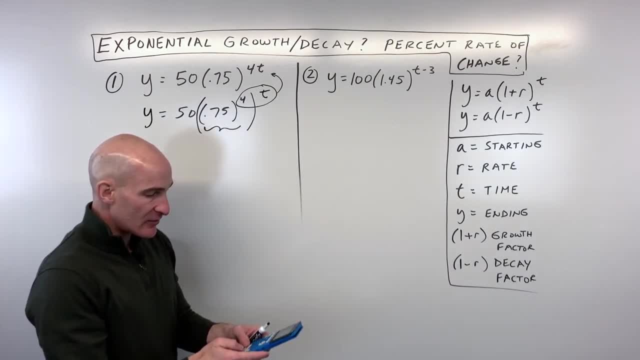 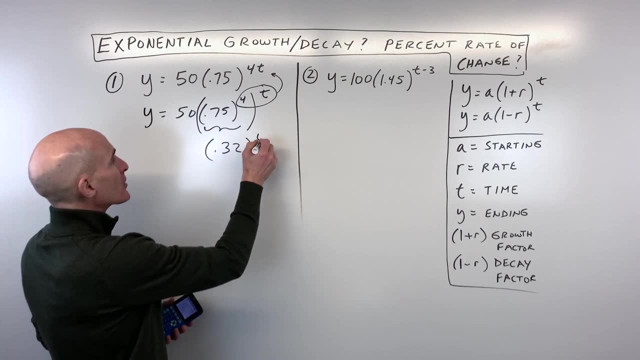 so let's go ahead and do that in the calculator. 0.75 to the fourth, I'm getting 0.32. I'm rounding a little bit here, so this is 0.32. check my work, if you'd like. and then now what you can see is we have. 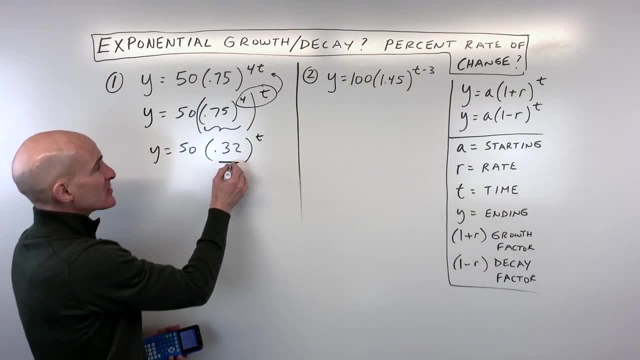 in our exponential form. here you can see this base: okay is 0.32. now, 0.32 is less than one, which we know. this is going to be an exponential decay function. the question is is: how much less than one is it? well, you could rewrite this further by saying: 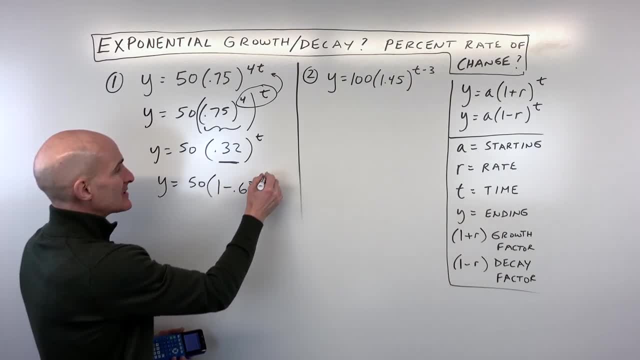 0.32 is 1 minus 0.68, and so now it matches this form right. here we can see that 50 is our initial amount and 0.68 is going to be our rate of decay, and I'm just going to take that 0.68 and move that. 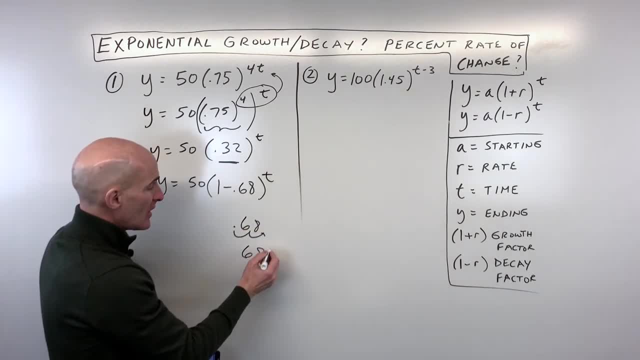 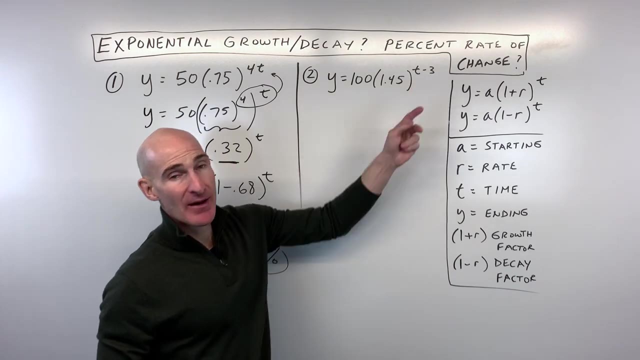 decimal two places to the right to convert this to a percentage and you can see that it's a 68 percent rate of decay. Let's look at another example, so number two. this one's slightly different. we've got y equals 100 times the quantity 1.45 to the t minus 3 power. again, it's not matching one of these two exponential. 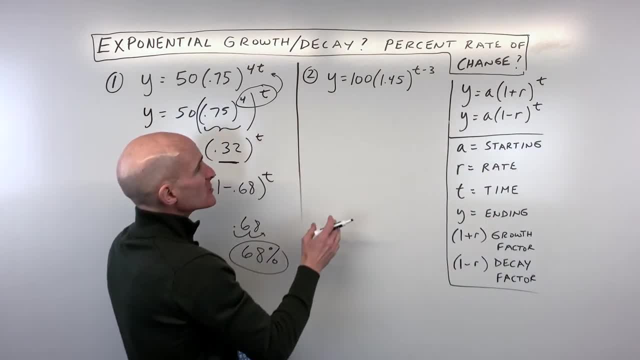 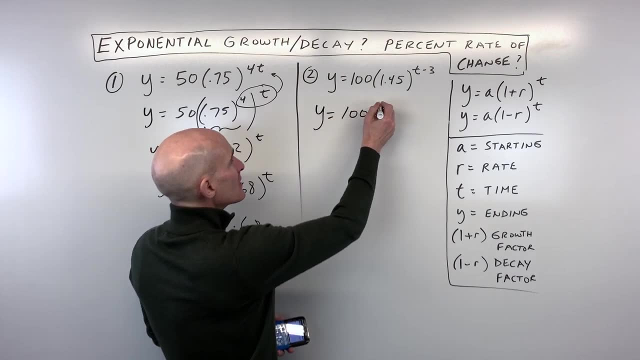 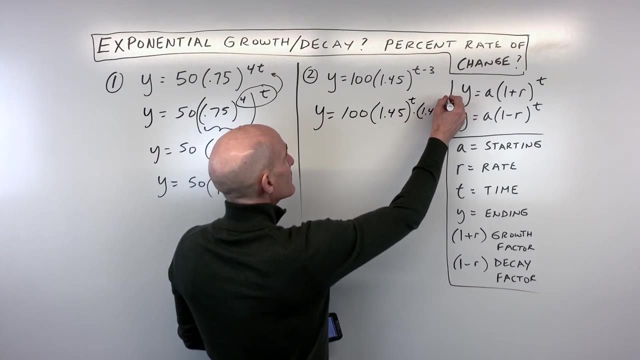 functions. so how can we rewrite it so it looks a little bit more closely like like one of those there? well, what I'm going to do is again using the rules of exponents: 1.45 to the t times, 1.45 to the negative. third, because remember, with the rules of exponents, when you're multiplying. 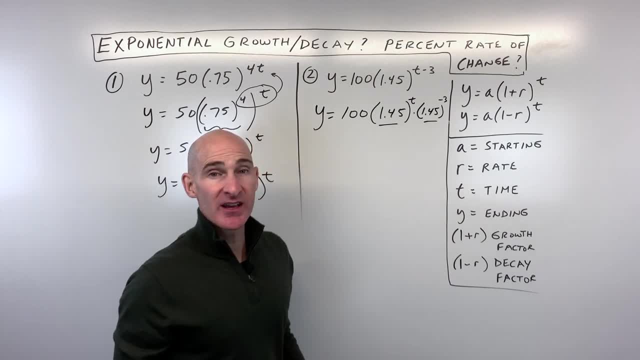 and the bases are the same. what do you do to the exponents? you add them, right? so in this case it's t plus negative 3, which is the same as t minus 3.. So we just rewrote it a little bit now I'm gonna. 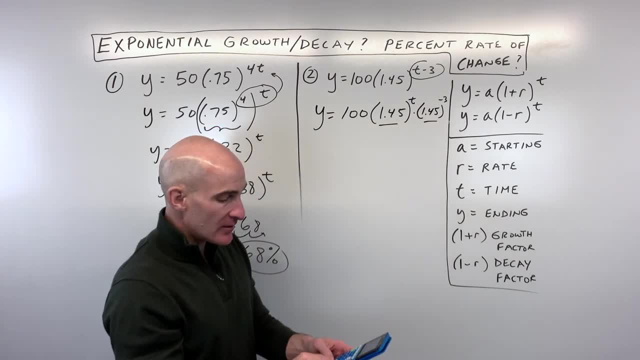 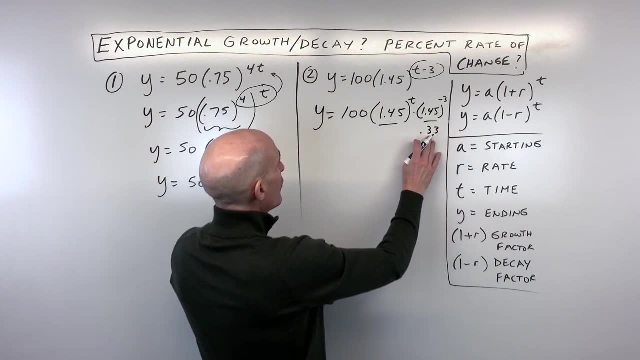 go to the calculator here and figure out what 1.45 to the negative third power is, and I'm getting 0.33 approximately, and I'm going to multiply that by 1.45- 100.. Now the reason I can do this is because see how all three of these groups are multiplied.